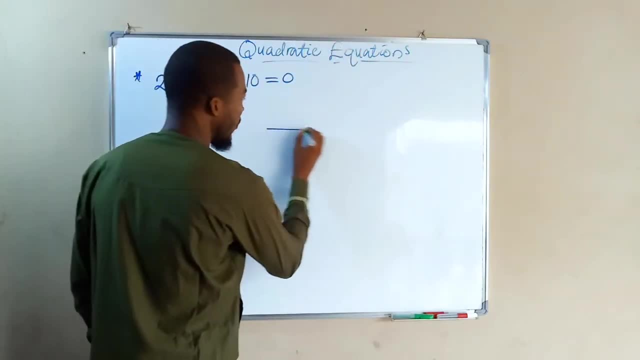 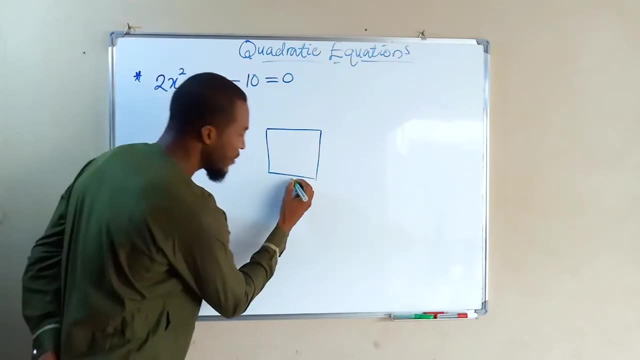 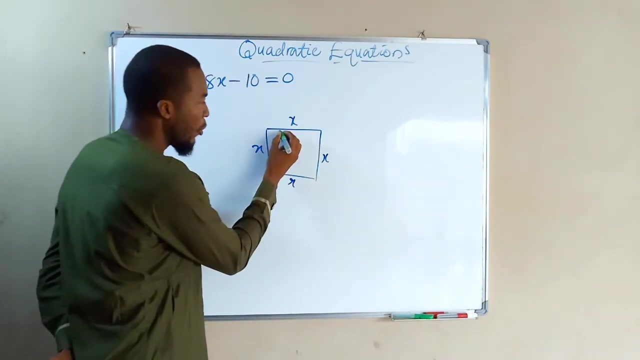 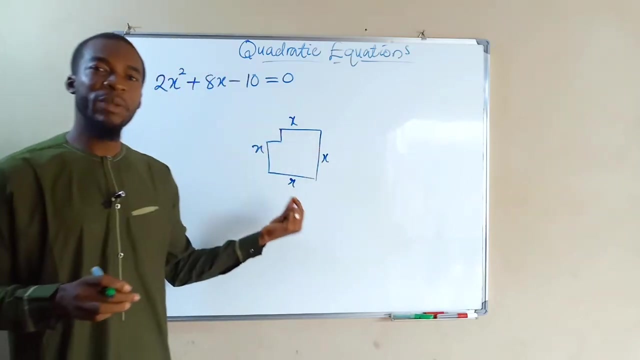 us to understand what it means by a square. a square is a plane figure that has equal dimensions. all sides are equal in a square, so if this side is x, all other sides will be x. but having a plane figure in this form, the square is not complete. to make this plane figure a complete square, you have to fill this. 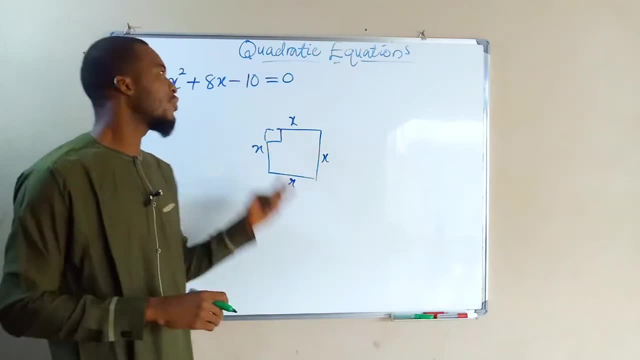 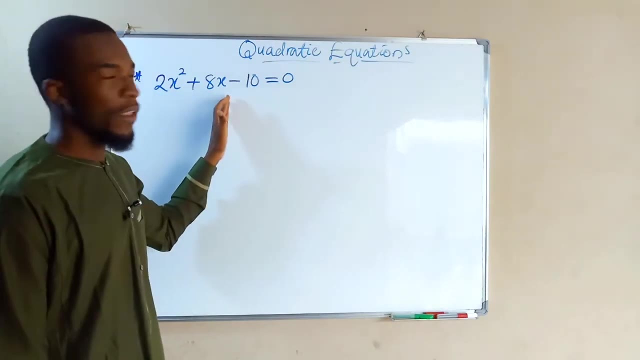 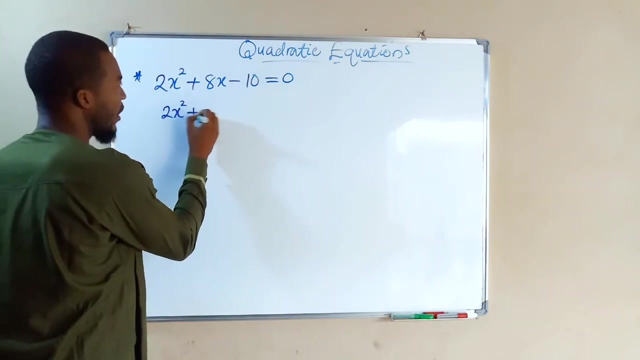 side and that's what we are going to be looking on to in this quadratic equation. in complete, in the square method, we only need the first and the second term. therefore, we are going to take the constant term to the right hand side, so we have 2x squared plus 8x from the left hand side. 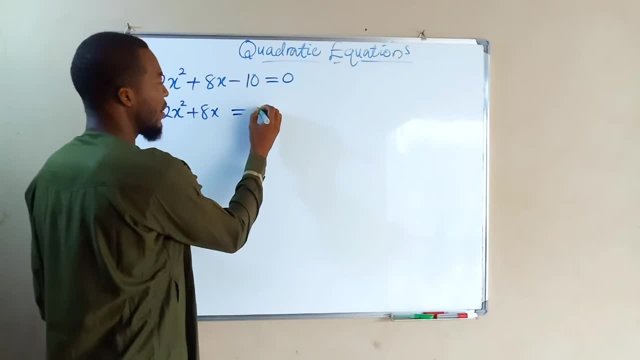 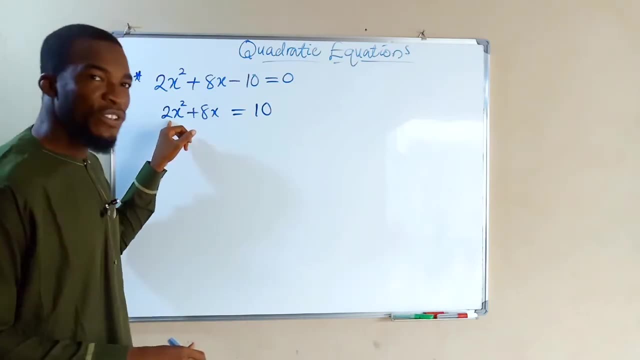 and to the right hand side. we are going to take negative 10 there and therefore it is going to become positive 10.. and always ensure that the leading coefficient is 1, but here we have it as 2, so we are going to divide both sides by this 2. 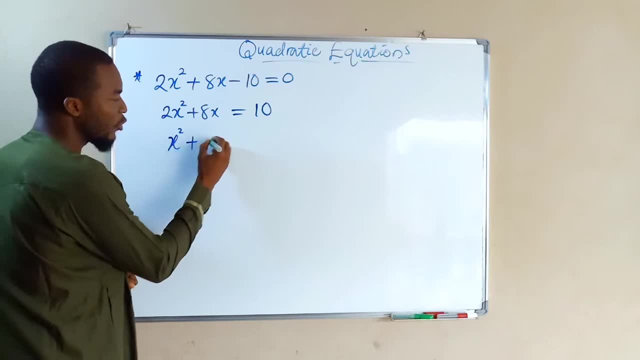 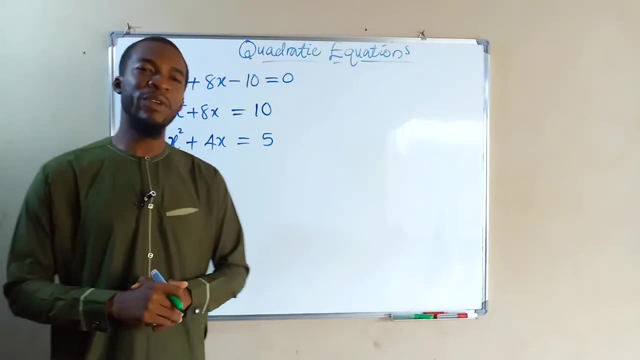 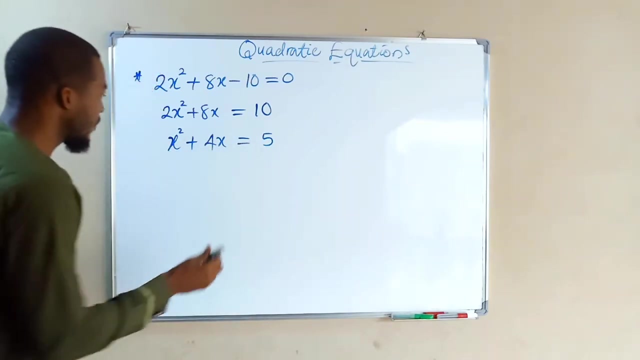 by applying these two scientific definitions. so the first term will become x squared, the second term will become 4x and the constant will become 5.. so now we are ready to complete the square. now we want to represent each of these terms by a plain figure. the first one is x squared, which. 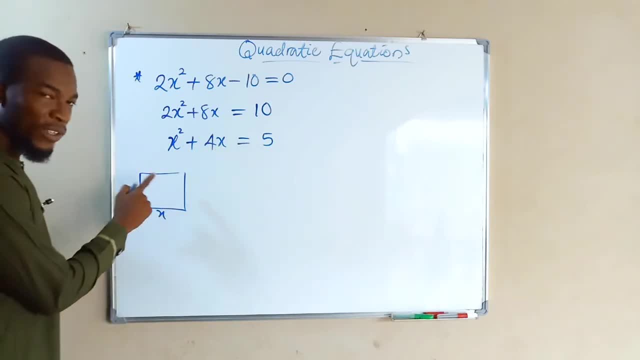 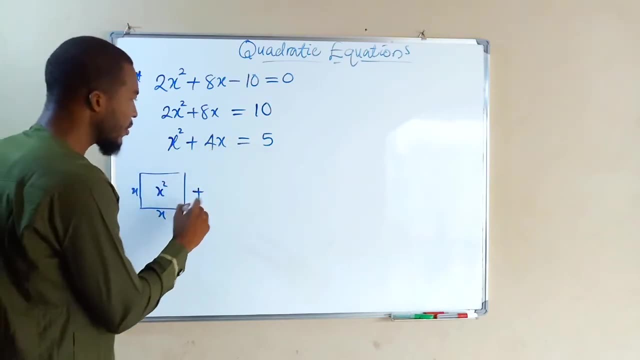 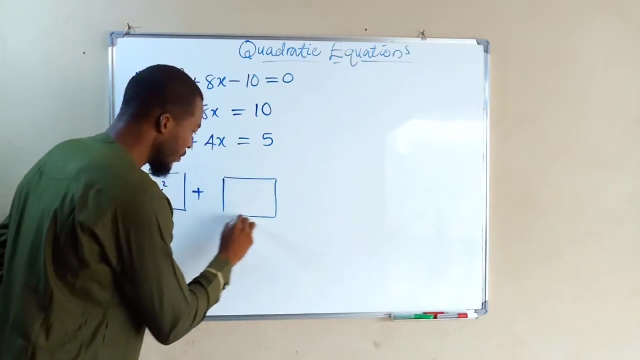 is going to be represented with a square of dimension x- X, Such that the area of this square is going to be x times x, which is x squared squared, which correspond to x squared plus 4x is going to be represented by a rect angle of dimension 4 and X, such that the area of this plane figure will 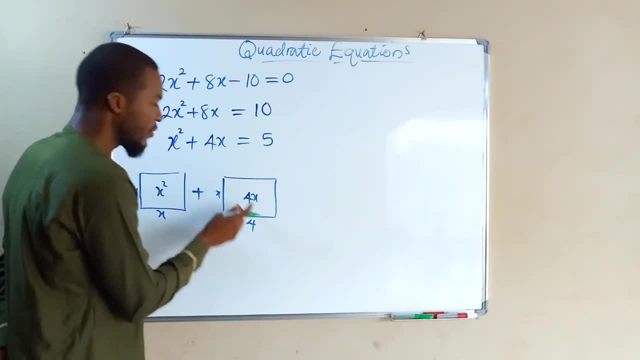 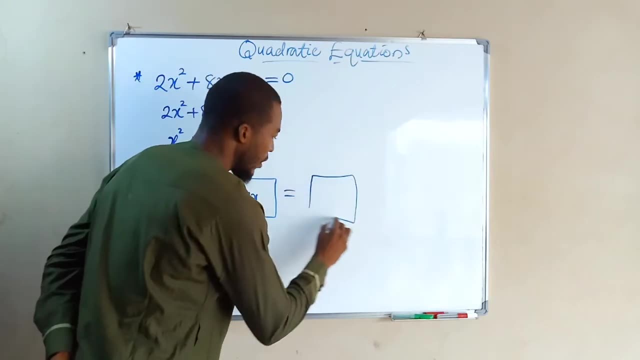 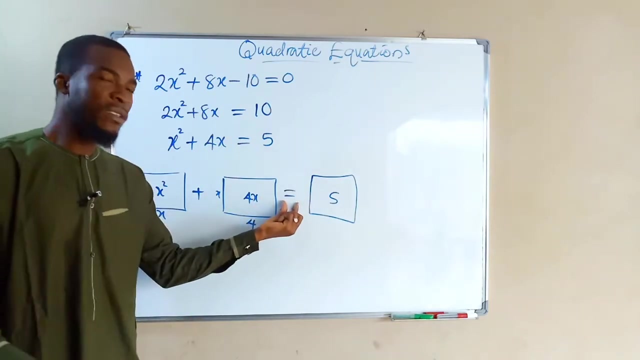 be x times 4, which is 4x. it also correspond to this 4x and to the right hand side we have a rect angle that represent 5 and the area of that rectangle is 5 units. equality sign is telling us what is on the right hand. 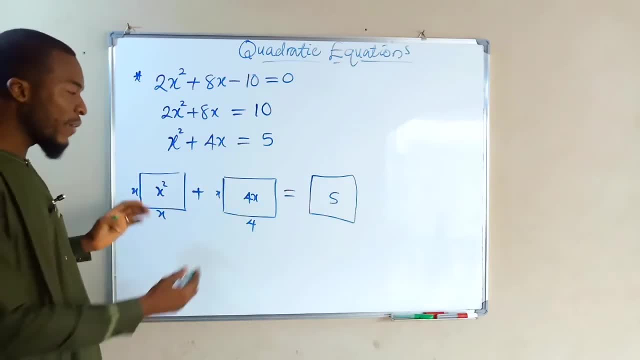 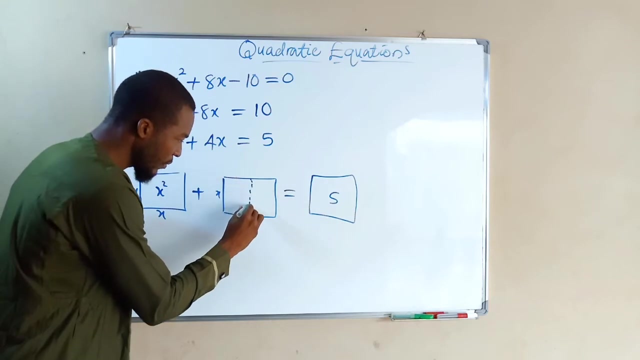 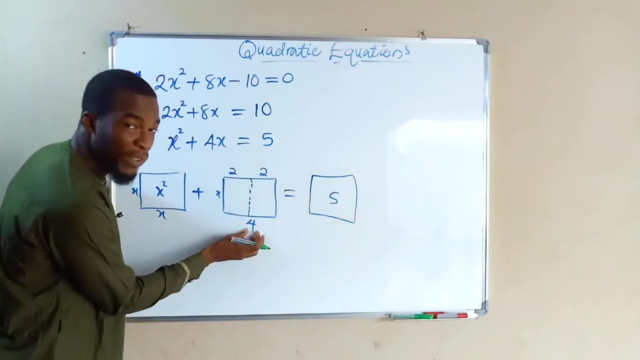 side is equal to what is on the left hand side. hence, we are free to add these two plane figures together and they will equal to the plane figure to the right hand side. so what I want to do here, I want to divide this plane figure equally, such that this side will become 2, and this side will become 2 because I have 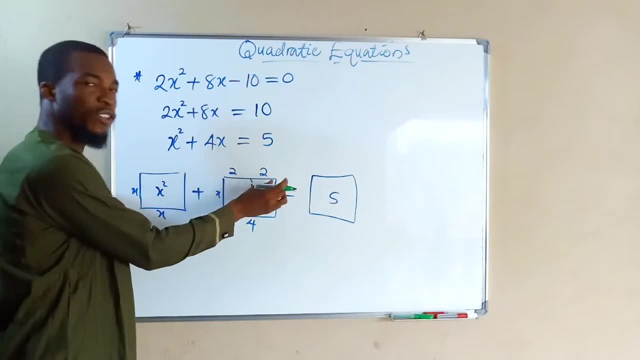 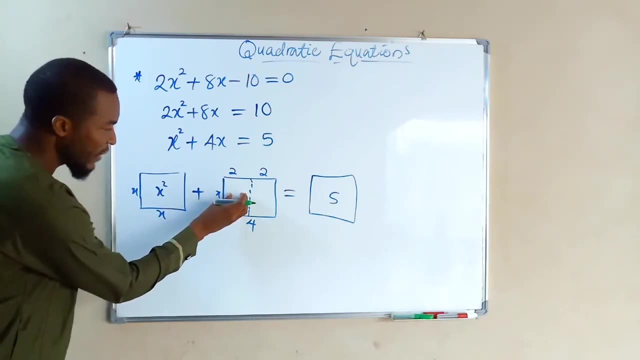 divided this length of 4 by 2, and each is equal to 2, and all other two dimensions remain X. what I want to do now, I want to take this side and connect it to this side and take the other side to this side. here is our 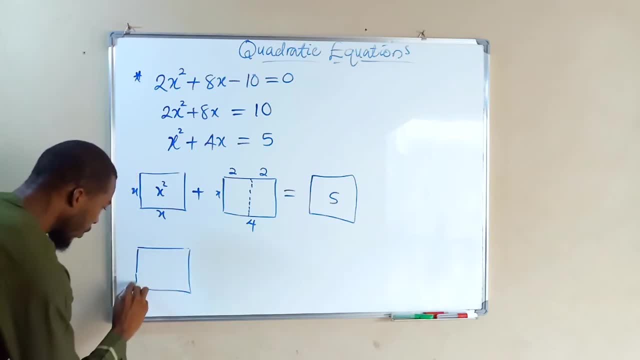 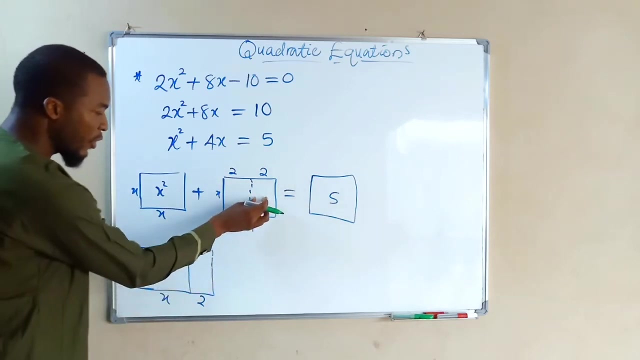 square of dimension X and X. now I want to bring this side to this side. already they have a corresponding side of X, so I don't have to write the X. this side is now going to be 2, while this remain X. now I want to connect this side to this side again. 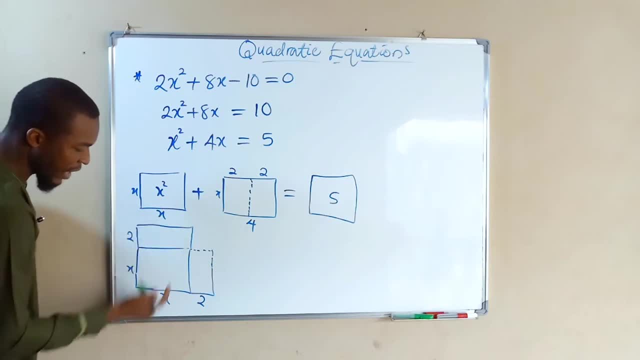 this side is 2 and this side remain X because it correspond to this length of X. if you look at this plane figure, it has a side length of X plus 2 and X plus 2, but this side is not up to X plus 2 because there. 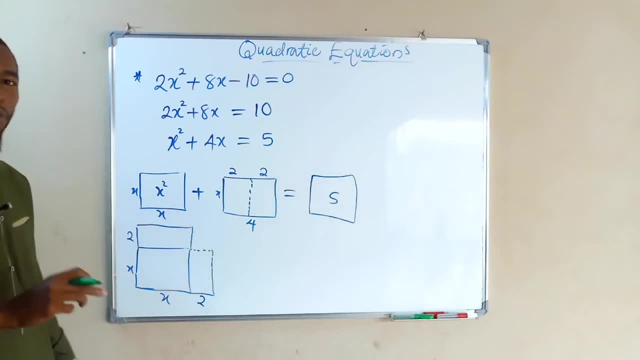 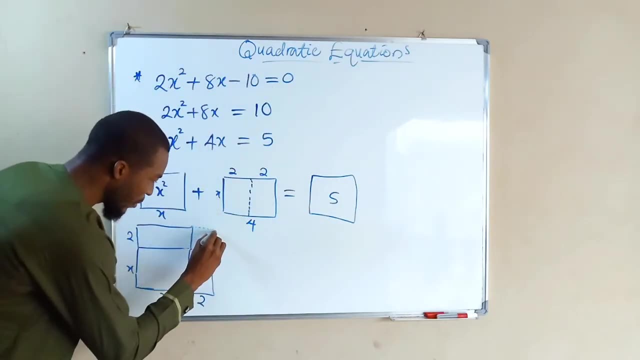 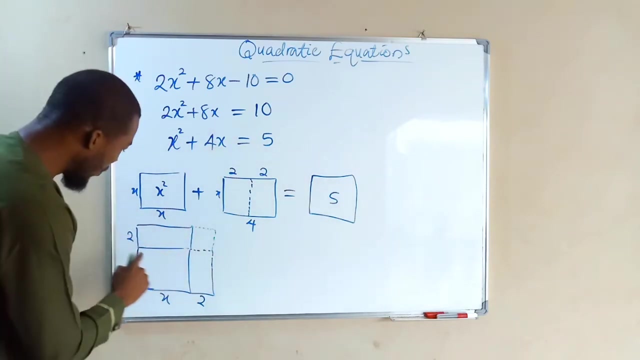 is a missing side here which we want to now complete. so to make it complete, to make it complete, we have to add a particular area here that will make this square a complete square. You know that the side length of this side is going to be 2, because it must correspond to this side. 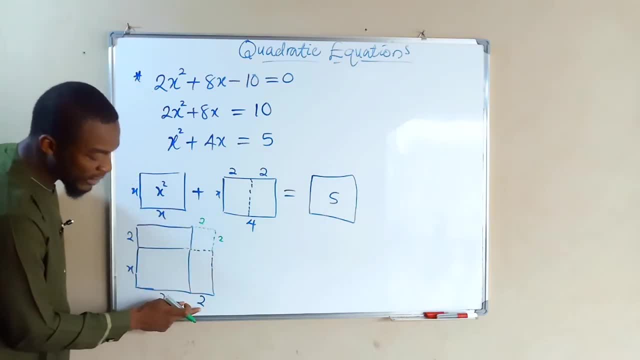 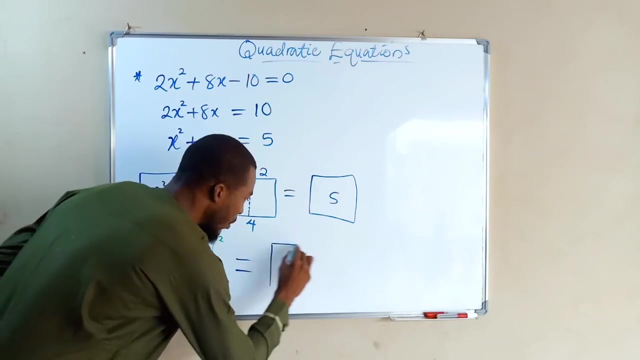 And the side length of this will now be 2, because it is going to correspond to this. Hence we say the total area added is 4, because 2 times 2 is 4.. And to the right-hand side we have our plan figure of 5 units. 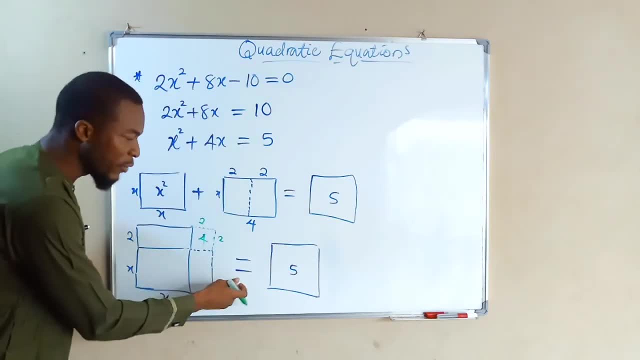 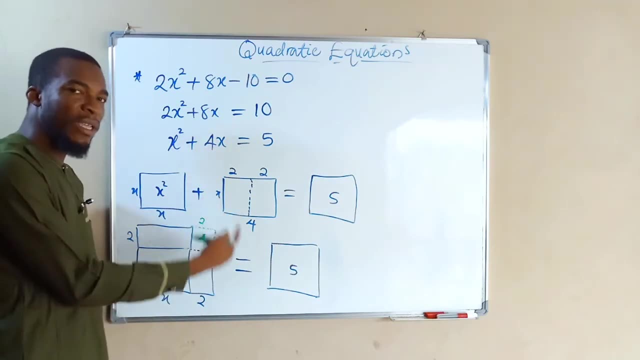 A quality sign is telling us what is on the right-hand side is equal to what is on the left-hand side, But from the left-hand side we have added 4 units To make the equation balance. we have to add 4 units here. 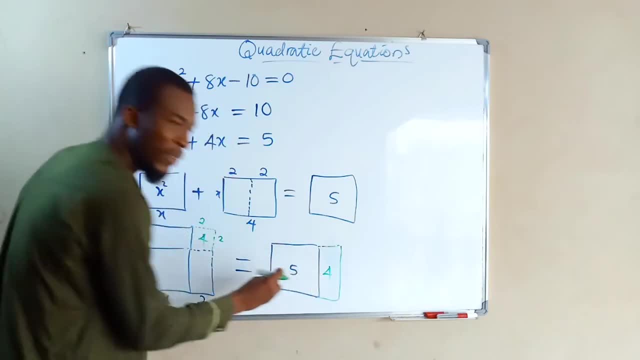 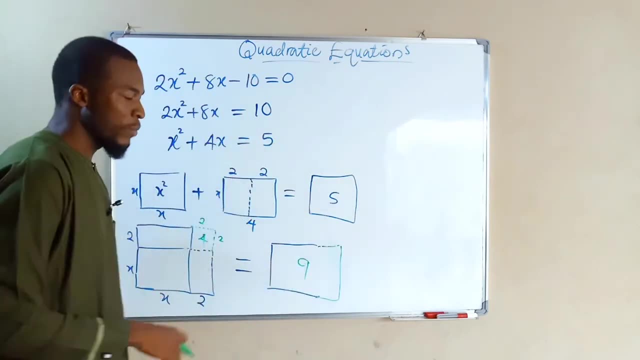 So we have 4 units. If you connect the two together we have 9 units. So I can clear here and write 9 units, A 9 unit, since it is an area, I can write 3 by 3.. 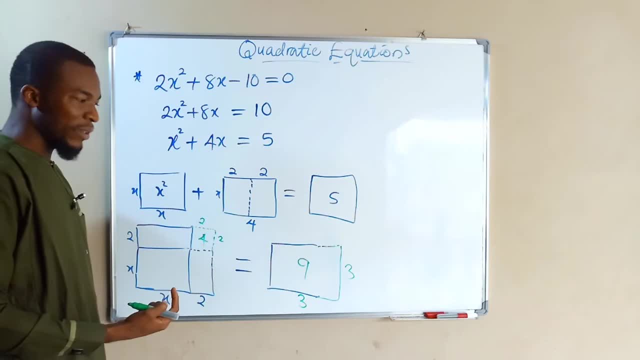 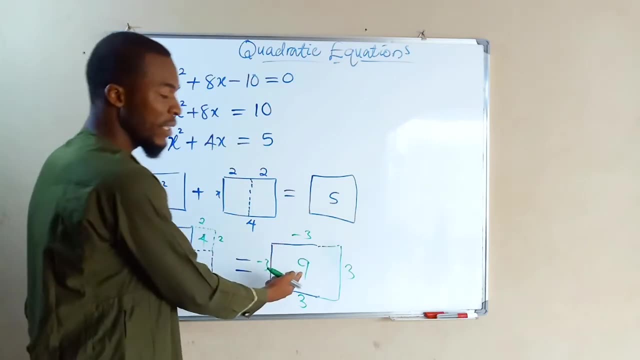 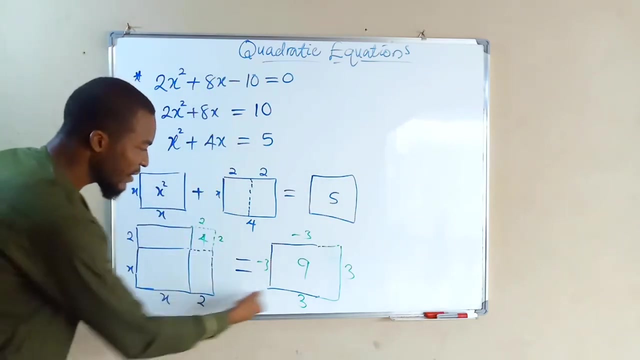 Such that 3 times 3 is equal to 9.. Or I can say negative 3, negative 3.. Negative 3 times negative 3 will still give me 9.. Now to find the solution for this quadratic equation. what we are going to do? we are going to relate the sides together. 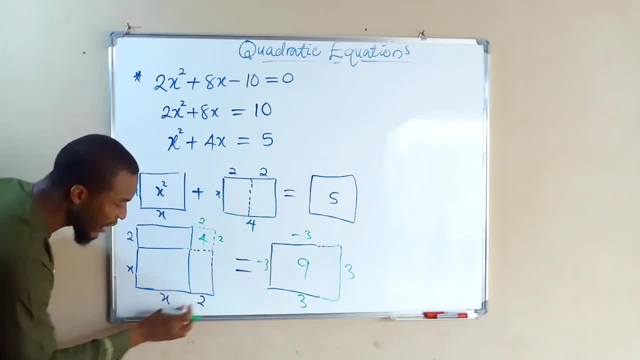 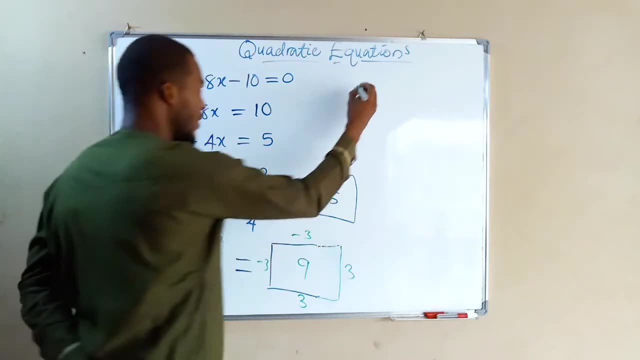 This side is x plus 2.. The total length of this side is x plus 2. And we have a total length of this side to be equal to 3. So we can equate them together. So we say x plus 2 equals 3.. 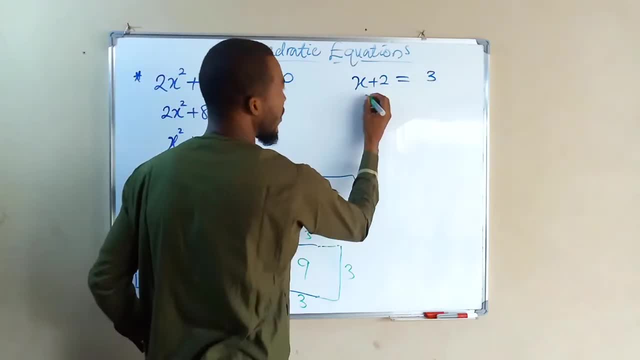 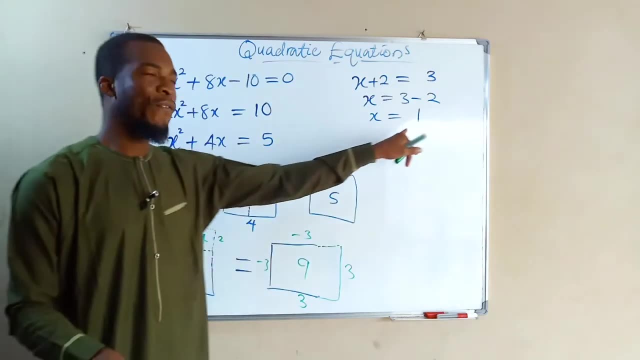 Now to find the value of x, we take 2 to the right-hand side And we say x equal to 3 minus 2.. And x is equal to 1.. We have found one of the solutions for this quadratic equation. To find the other solution we can relate the other side again. 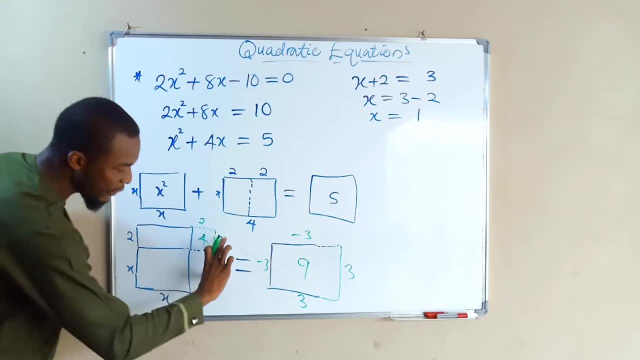 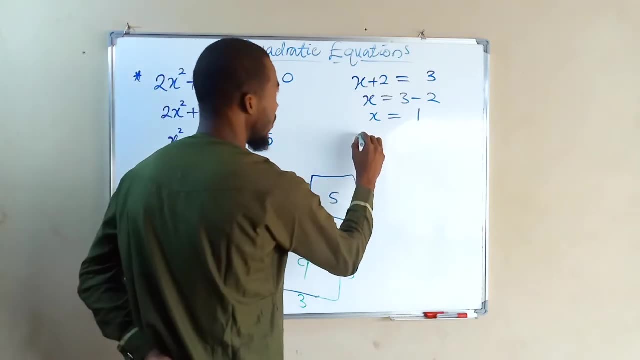 You can see that this side is x, This side is 2.. If you add them together you get x plus 2. And you can relate it with this negative 3.. So we can say: x plus 2 is equal to negative 3.. 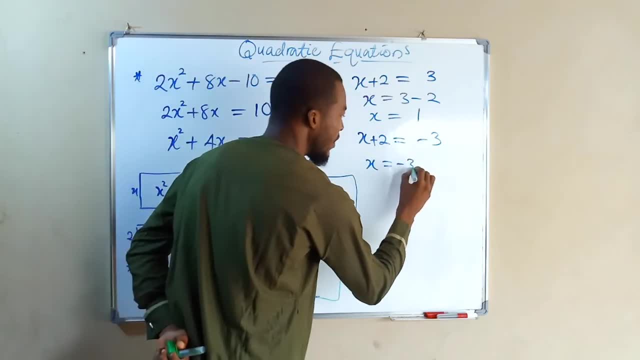 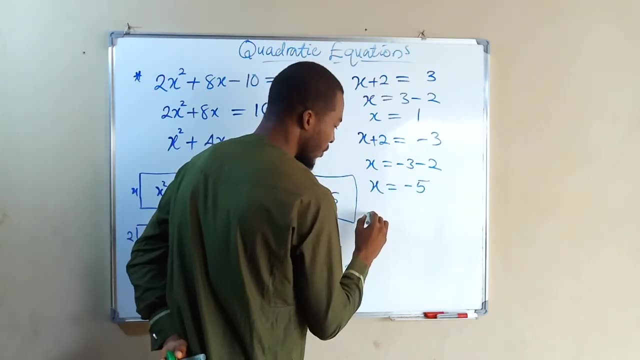 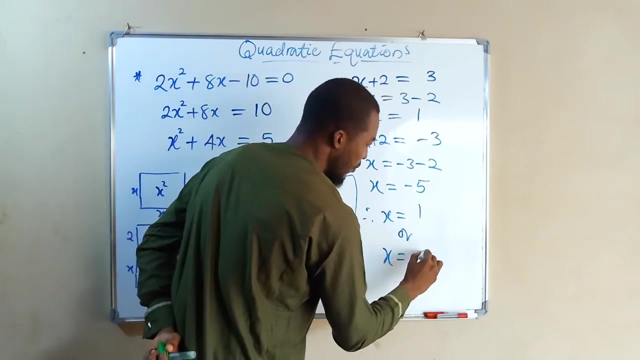 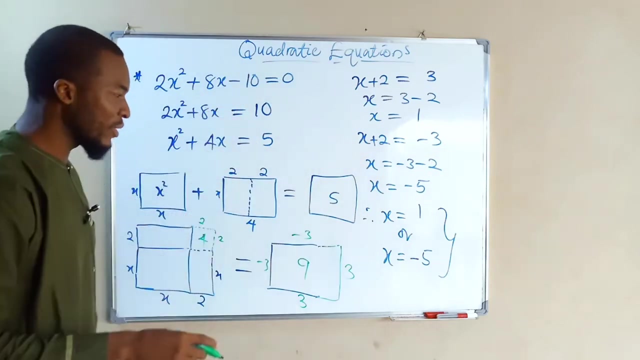 x. if 2 crosses over, we have negative 3, negative 2. x will now be equal to negative 5.. Hence we say x is equal to 1.. Or x is equal to negative 5.. Hence 1 and negative 5 are the root of this quadratic equation. 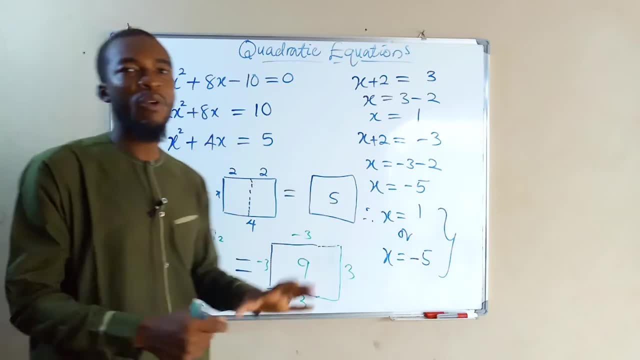 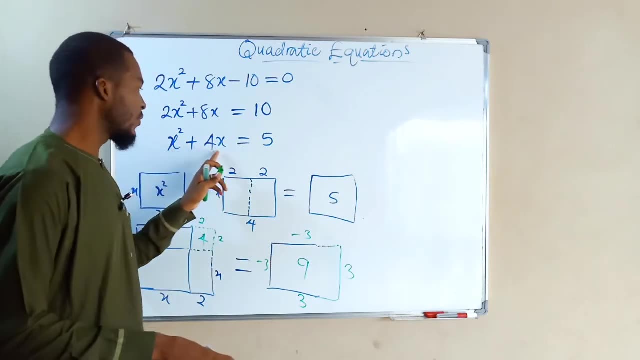 So, geometrically, this is how to solve quadratic equations: by completing the square method. So let me explain all this mathematically. This is the equation we have: x squared plus 4x is equal to 5.. x squared plus 4x is equal to 5.. 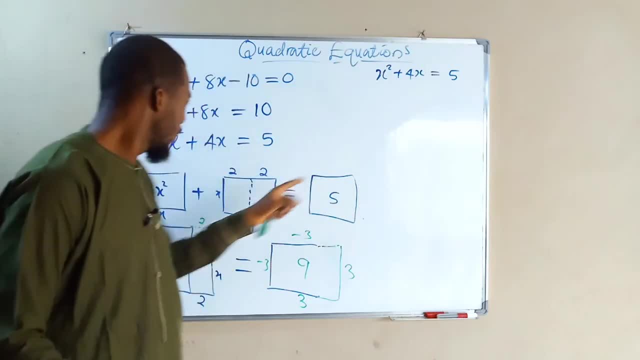 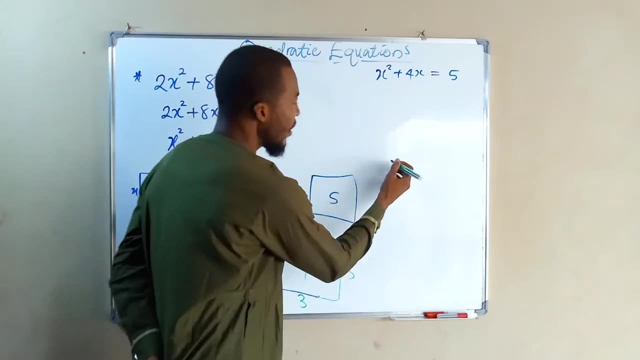 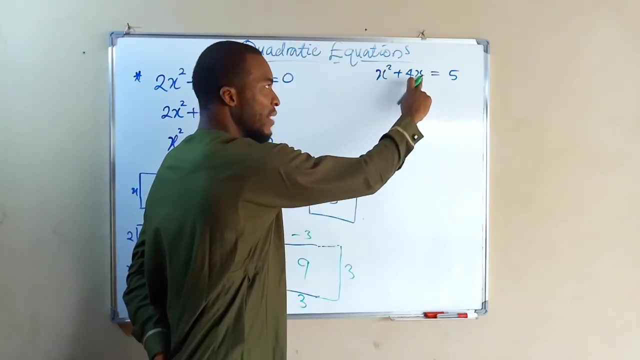 To make the left-hand side a complete square. this is what we have added 4.. And how do we get this 4?? 4 is just half of the coefficient of the middle term, And the middle term is 4x And the coefficient of the middle term is 4.. 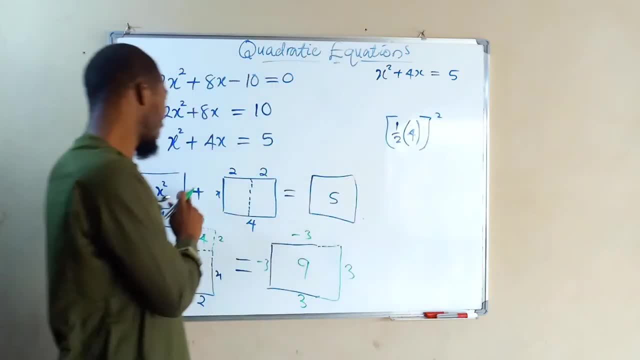 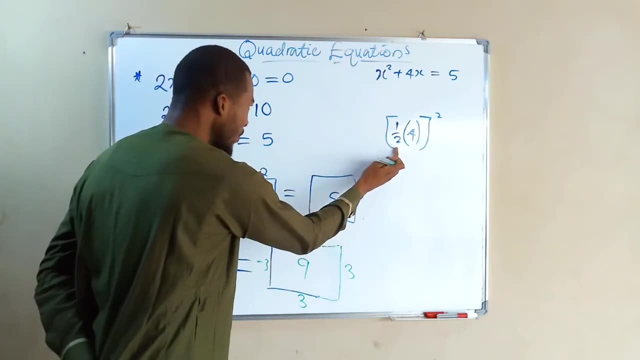 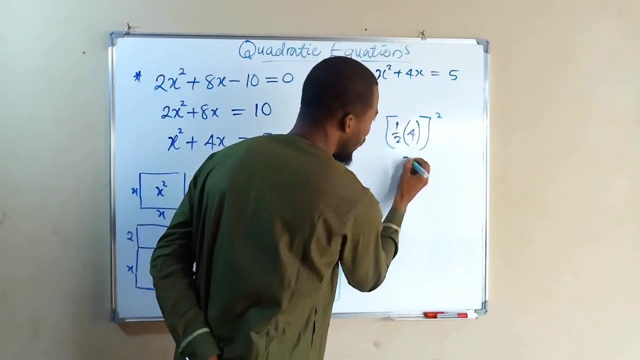 All squared. This is what we have added here, Because, you see, we divided it into 2, which is half, And we get 2.. Then we square it and we get 4.. So half of 4 is 2 squared. 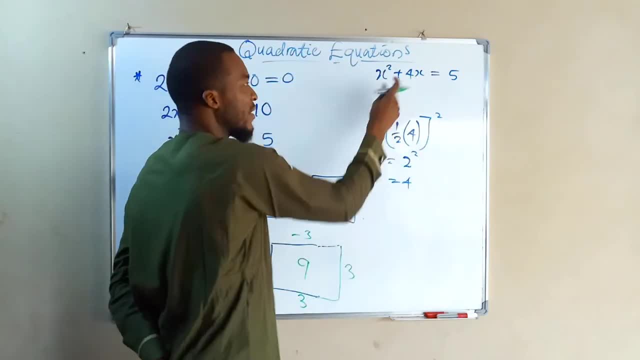 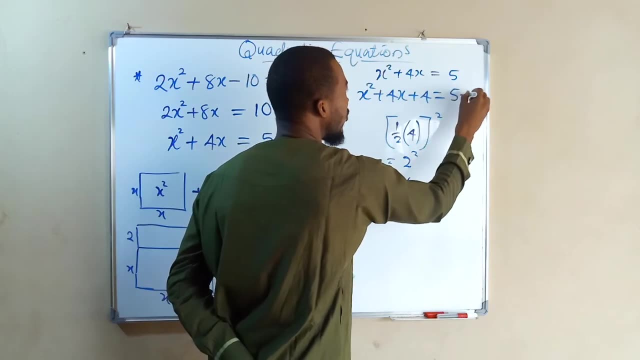 And this is equal to 4.. So we are going to add 4 to this side, so that we have x squared plus 4x plus 4 is equal to 5 plus 4. because we don't have 4 initially, We added 4.. 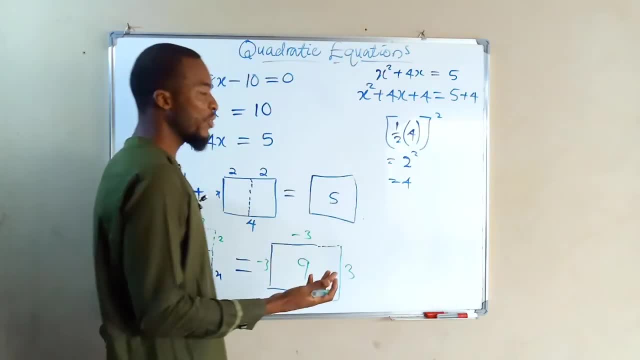 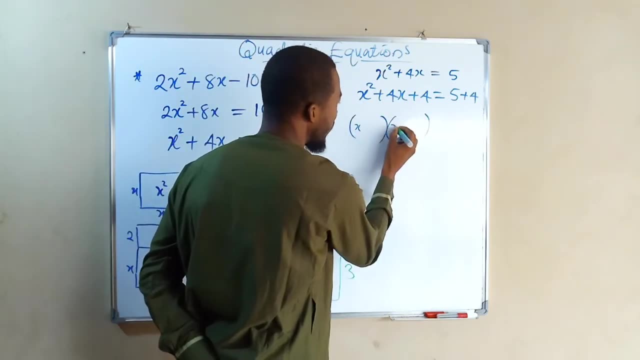 Therefore we have to add it to the other side in order to make the equation balanced. So let us factorize this one. We have our brackets, We have our x's. Think of two numbers which, when you multiply them together, you get 4.. 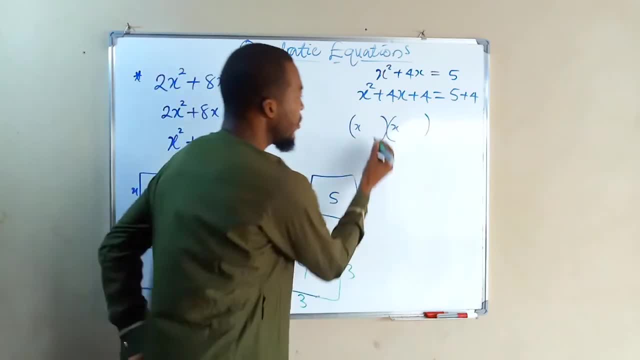 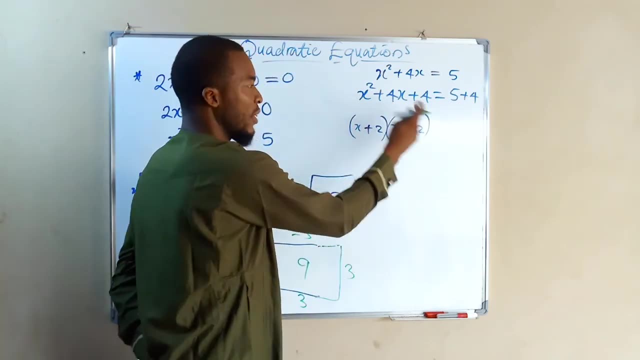 And when added off together, it equals 4.. The numbers must be 2 positive and 2 positive, Because 2 times 2 is 4. And 2 plus 2 is 4. And to the other side we have 9.. 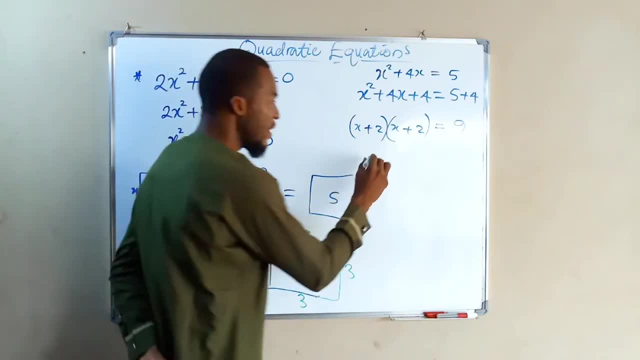 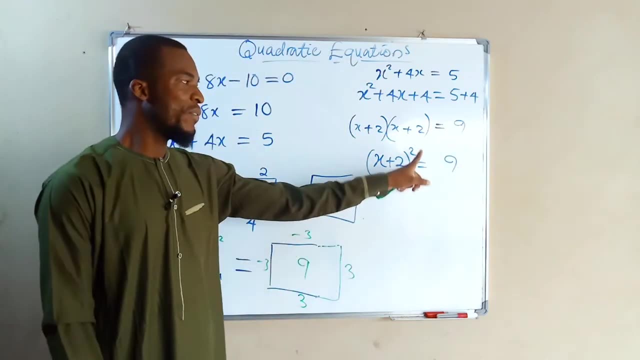 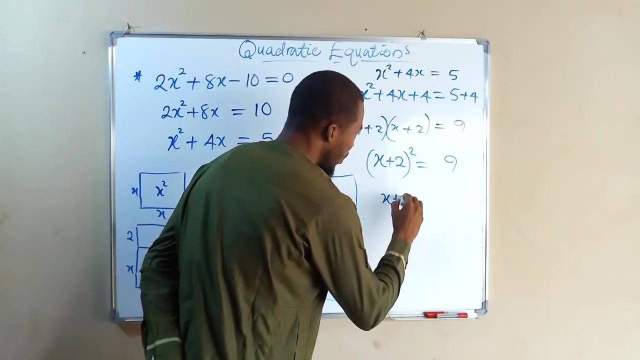 If you look at these factors, they are the same. So we can say x plus 2 squared equals 9.. To remove this, we are going to take the square root of both sides of this equation, Leaving only x plus 2 to the left-hand side. 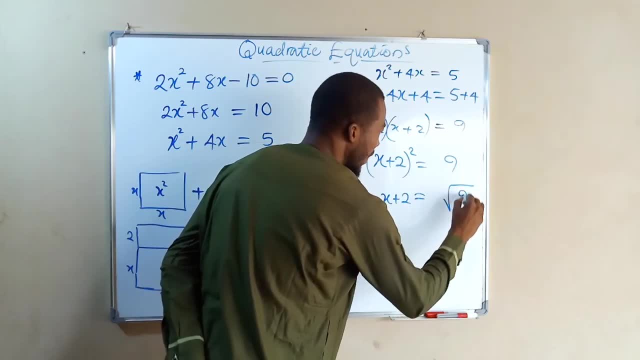 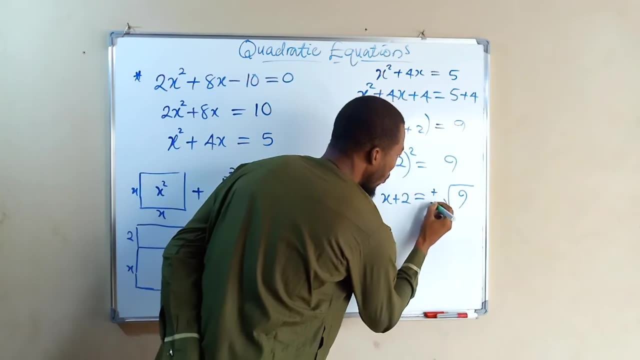 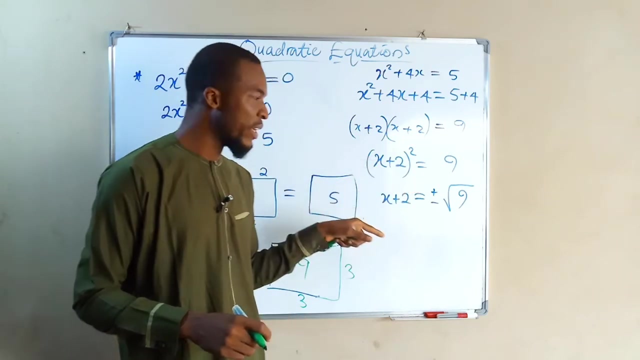 And to the right-hand side we have a square root of 9.. But remember, in one of my videos I explained to you why we always have plus or minus Once you introduce a square root to a number that does not have a square root initially. 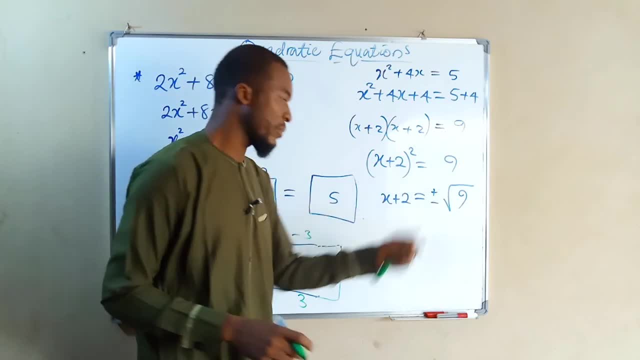 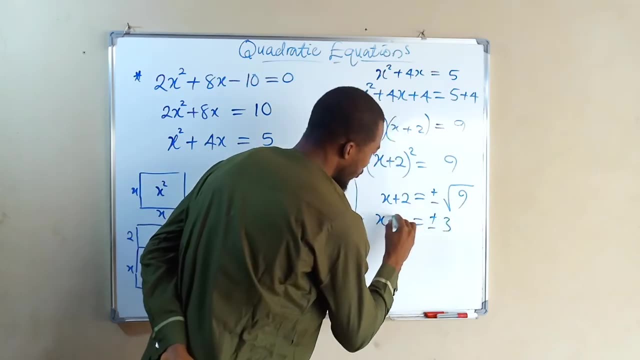 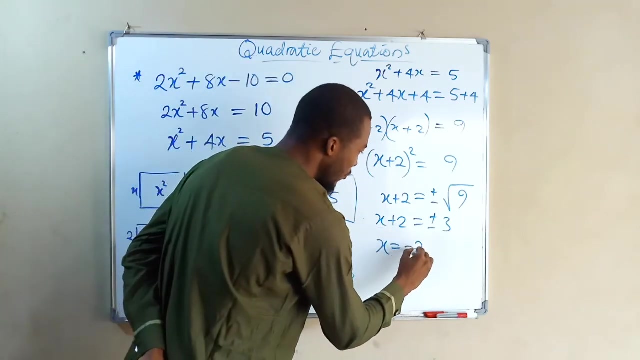 you have to introduce plus or minus. Square root of 9 is 3.. So we have plus or minus 3. And this is x plus 2.. x is equal to: if 2 crosses over, it becomes negative: 2, plus or minus 3..